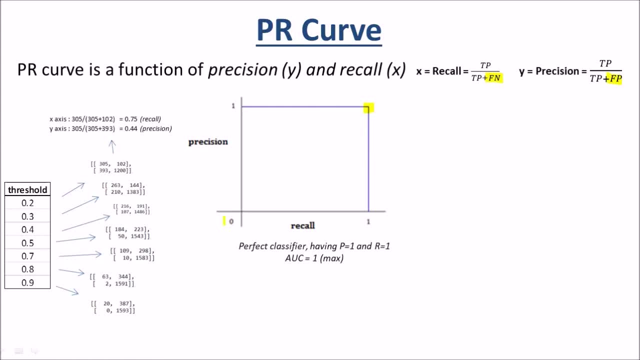 from 0 to 1. my area under the curve is 1 square unit or just 1, so my maximum AUC can be 1. now you must be wondering: when can this be the case? well, just imagine if i have 6 people in the test set and out of those, the first 3 people do not have a particular disease. 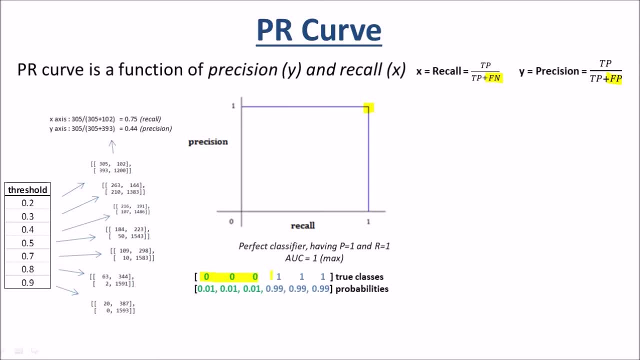 if we are talking about a medical case scenario and the next 3 people have a disease? ok, so these are 1s and these are 0s. now, if my model is so good that it is predicting for the first 3 people that they have only 1 case scenario and the next 3 people have a disease, ok, so 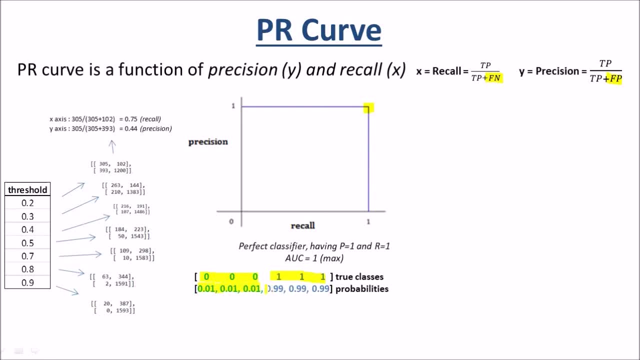 these are 1s and these are 0s. now, if my model is so good that it is predicting for the first 1 person chance of having the disease and these people, the next 3 people, they have 99% chance of having the disease- then a model is basically very good. right then at any particular. 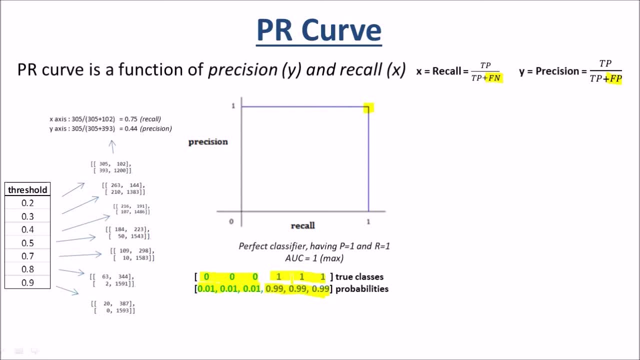 threshold value. if you check a model will not make any mistake. so, and hence i'll have precision equal to 1 and recall is equal to 1. now when i say at any particular threshold, basically under the hood, the thresholds will be chosen by looking at the unique number. 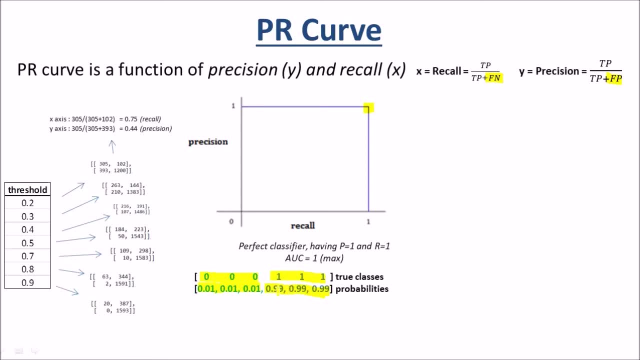 of probabilities. ok ……ک. So I have only two unique probabilities here of 0.01 and 0.99.. So these will be the two threshold values which will be chosen for creating the confusion matrices. So I'll have two confusion matrices and the precision recall curve will be drawn in that way. 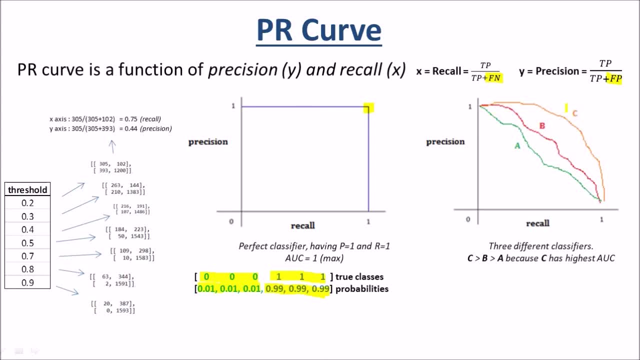 Now, if I have three different classifiers, okay, So my classifier C will be the best one out of these because it has the highest area under the curve and also it is closest to this point of 1,1.. So the closer a classifier is to this point of 1,1,, the better it will be. 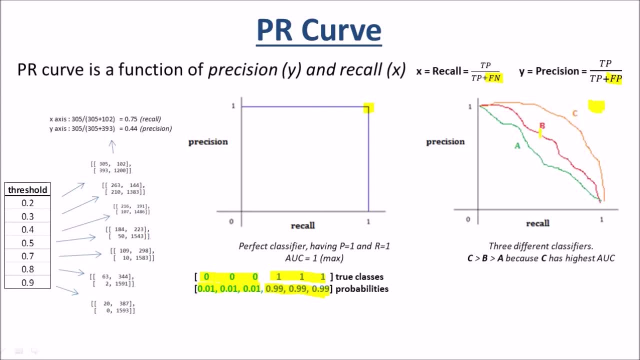 So my classifier A will be the worst one and B will be the middle ground between C and A. Now the baseline PR curve area under the curve is given by the total number of positive samples in the data divided by the total number of data samples which I have in my data. 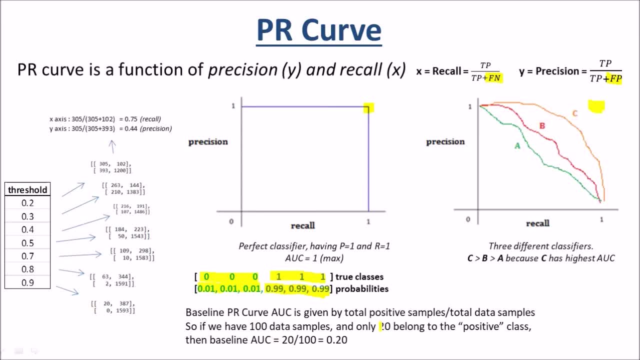 So if I have 100 data samples in my test set and only 20 of them happen to belong to the positive class, then my baseline AUC will be 20 by 100, which is 0. So with this 20% I can judge my classifier whether it is any good or not.